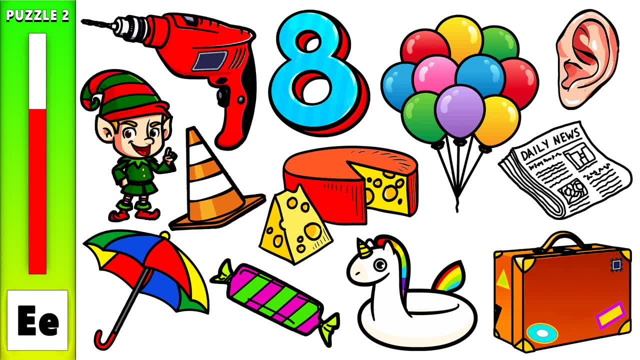 2, 0, 3 & 2, 5, 6-ồ 1, 6-ồ 7, 3 & 2, 4 O 3, 2, 1, 1, 2, 2, 1, 2, 2, 2. 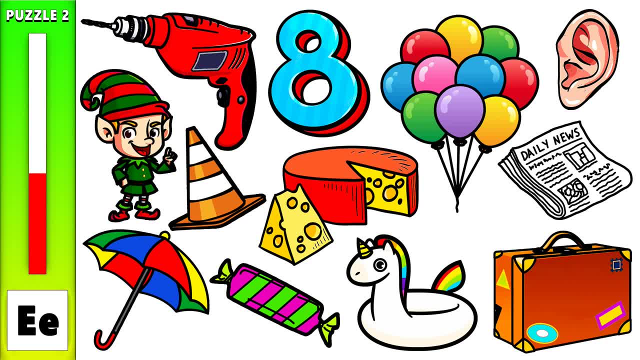 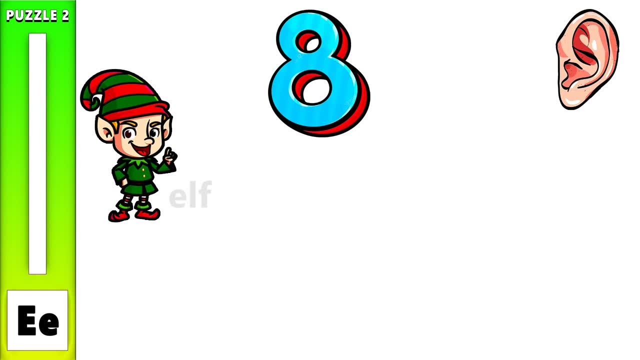 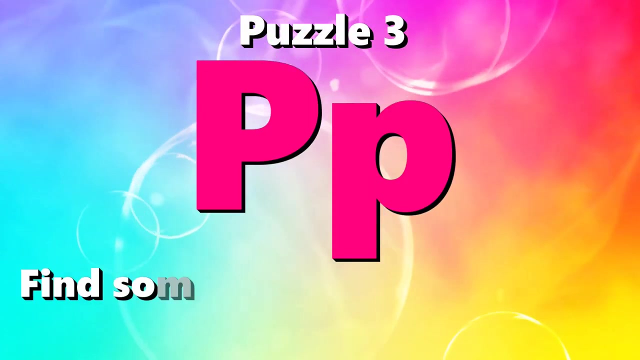 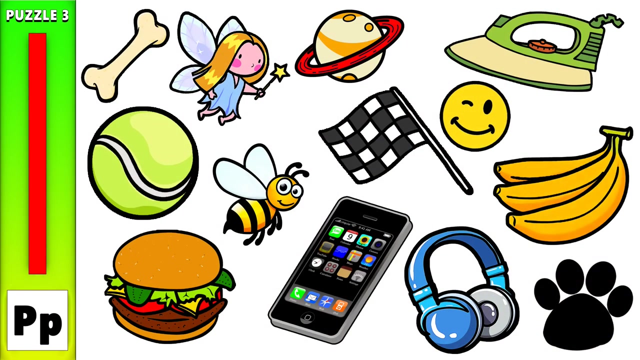 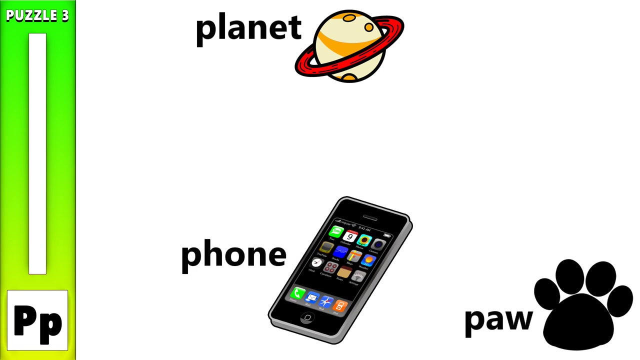 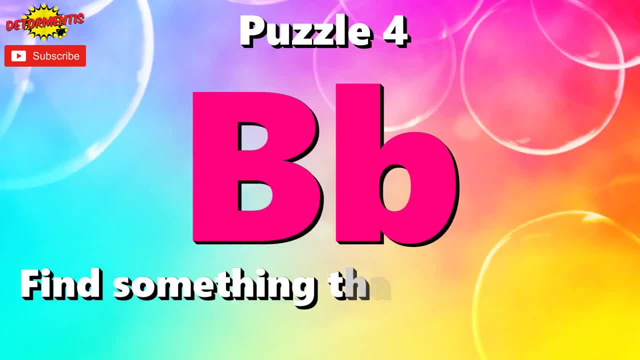 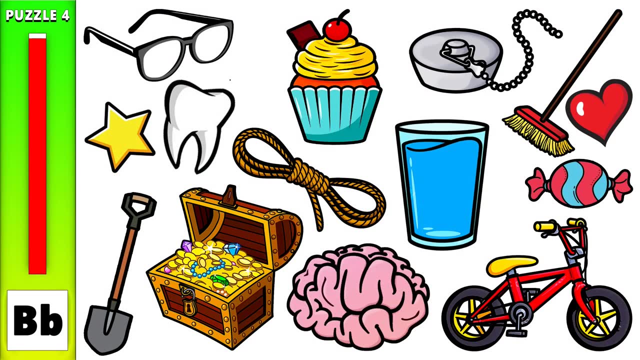 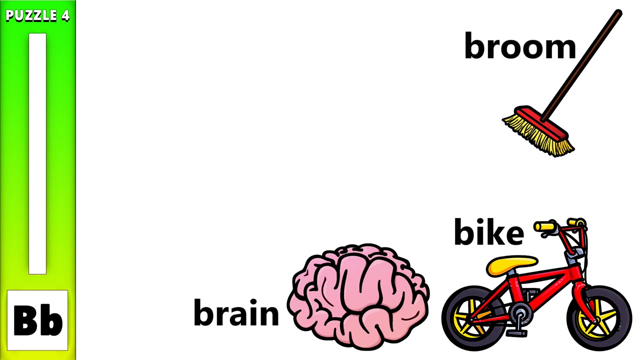 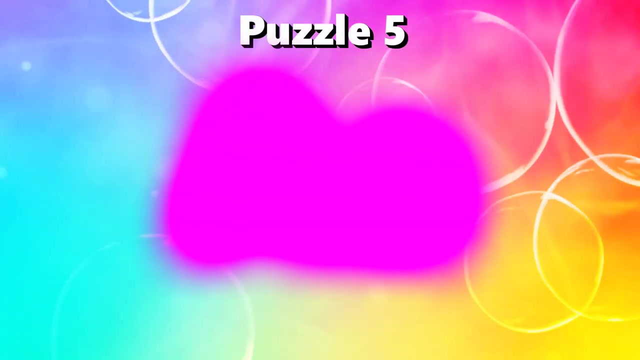 I spy with my little eye something beginning with the letter B- P-P-L- something new name name: Merong 🤟. P-P-L 7, P-P-L. Kl. Cl Brain Bike Broom. I spy with my little eye something beginning with the letter A. 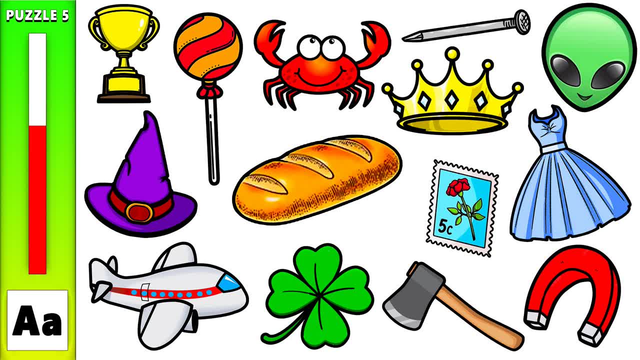 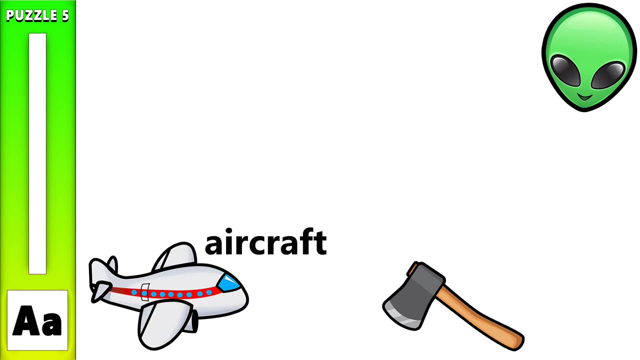 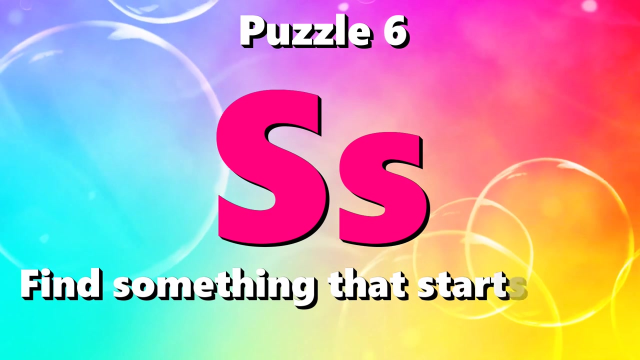 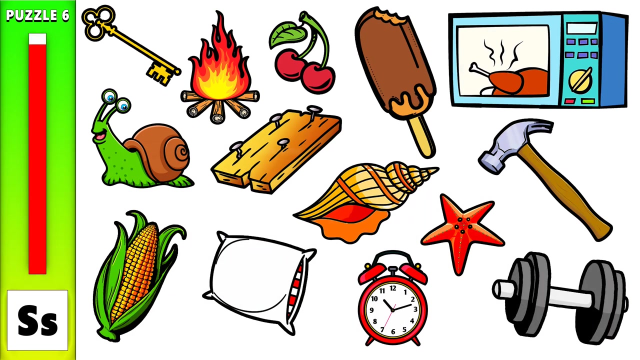 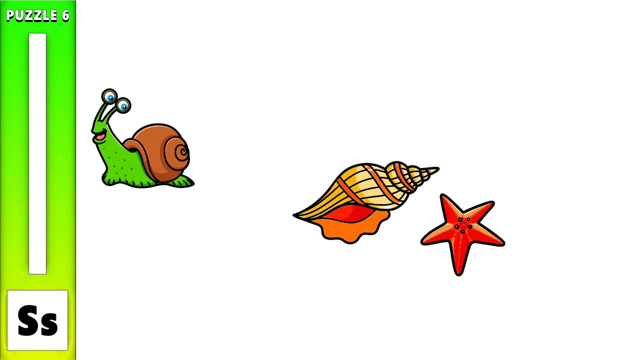 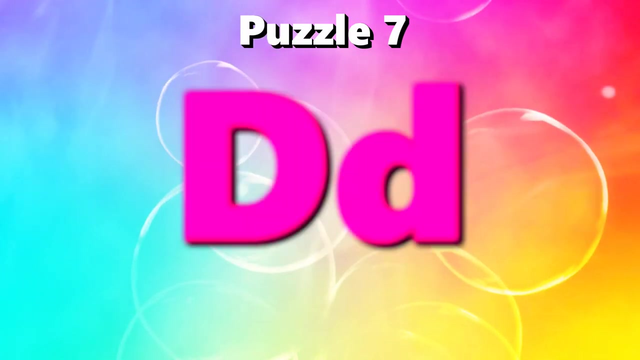 Aircraft Axe- Alien Puzzle number 6.. I spy with my little eye something that starts with an S- Snail Shell Starfish. I spy with my little eye something that starts with an E. I spy with my little eye something that starts with an E. 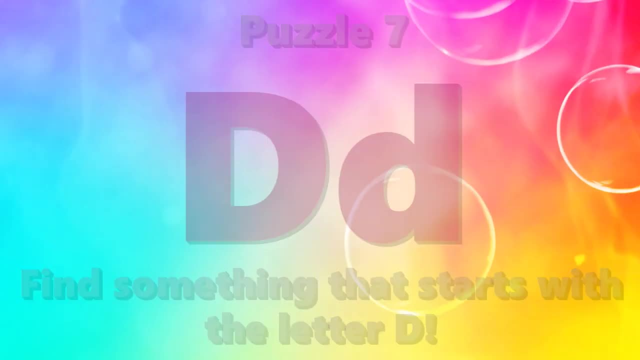 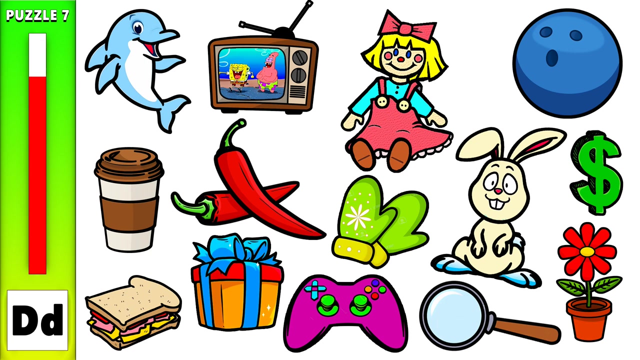 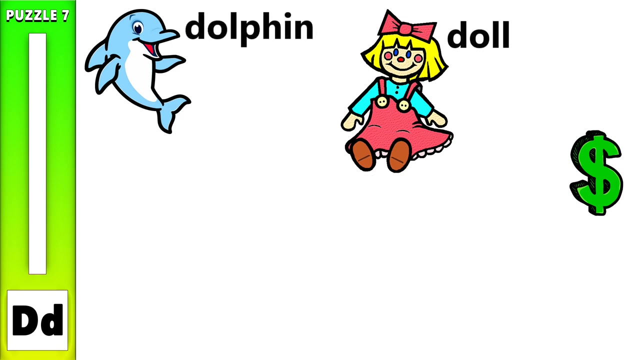 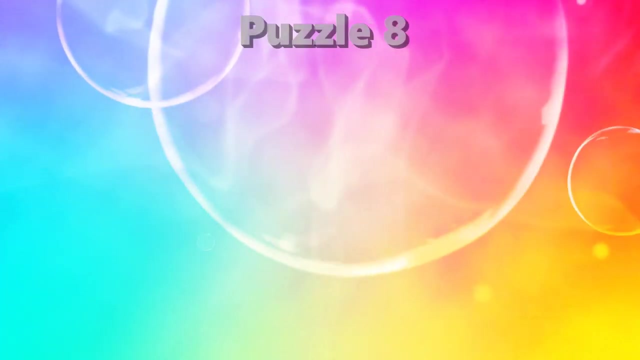 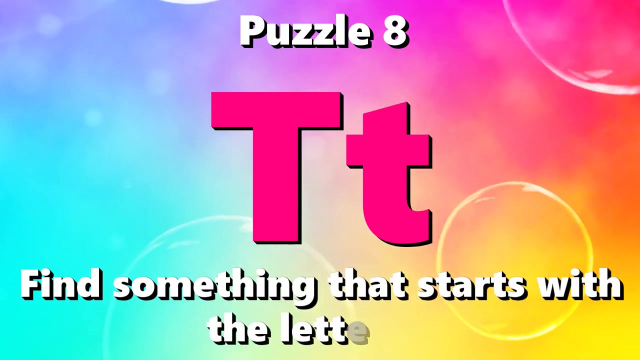 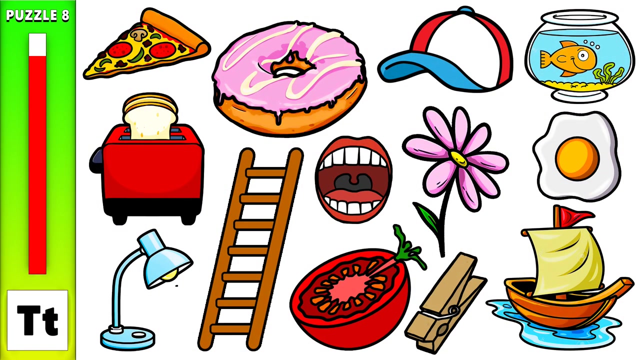 I spy with my little eye something that starts with an E- Dolphin Doll, Dollar, Puzzle number 8.. I spy with my little eye something beginning with T, getan необход Liberia, Puzzle number 9.. I spy with my little eye something that stopped with the letter X. 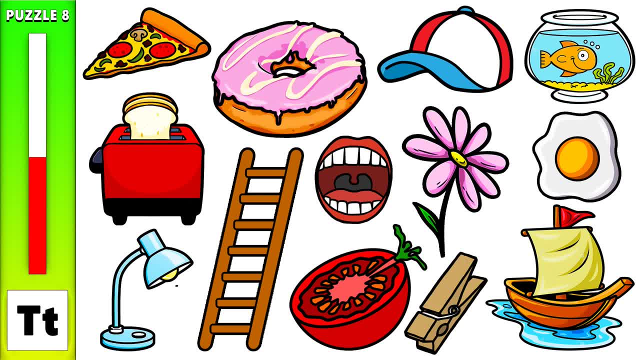 Aенная Отelorda. I spy with my little eye something with a Mustafa tongue. I spy with my little eye something that starts with a C Milrt. I spy with my little eye something that starts with a P Toaster.